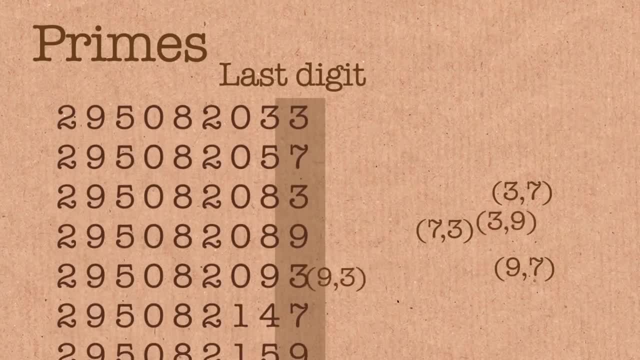 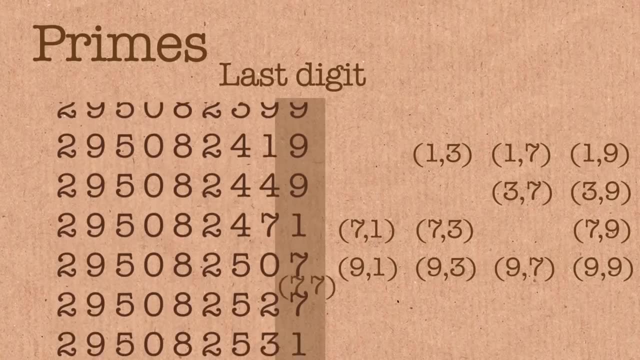 followed by a three Or one, followed by seven, Or one, followed by nine, And these are the options. okay, There are 16 options when you're looking at two consecutive primes. So if it was random, they should all appear one-sixteenth of the time, equally likely of the time, But that's. 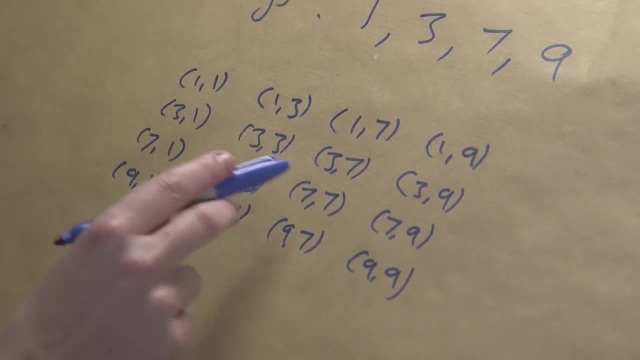 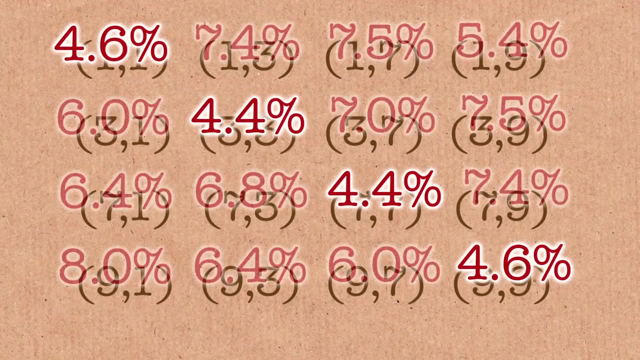 not what they found at all, In particular these diagonal entries here. so the one, one, three, three, seven, seven, nine, nine are least likely to turn up. So the primes aren't repeating themselves. And there's a few. 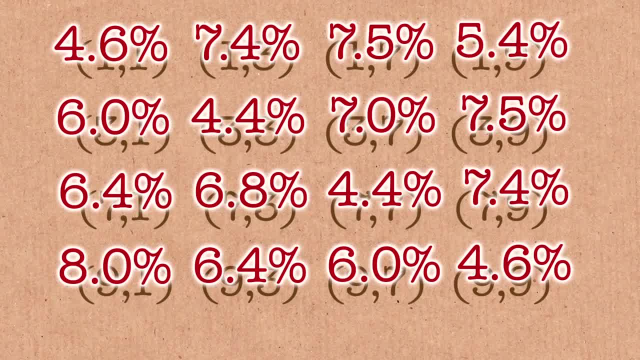 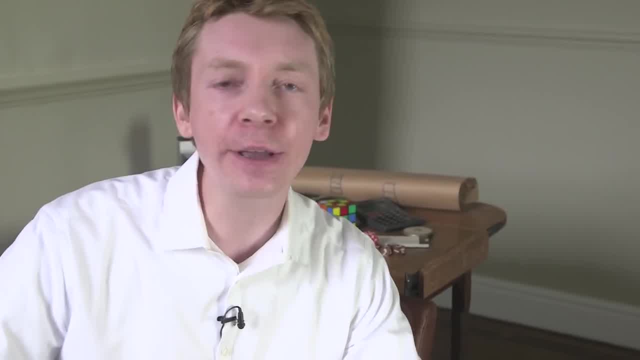 explanations for why this could be the case, which I'm going to dismiss. all right, I'm going to give you a few explanations which aren't the reason why this is happening. So one might be okay. if you have a prime ending with a nine, then well, you have to go through all the other numbers. 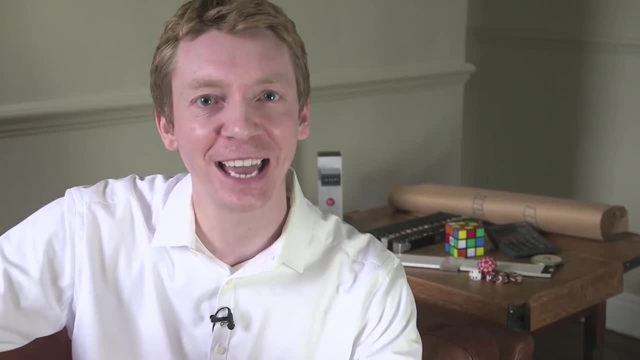 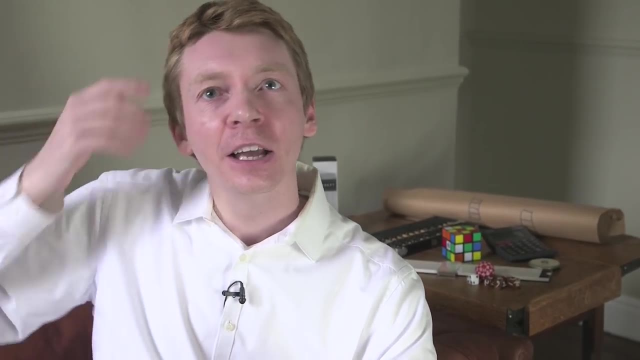 before you get to another prime ending with a nine, Or you have to go through the numbers that end with a one and a three and a seven before you get to another number ending with a nine. It's further away. It's further away, right? So unfortunately that's. 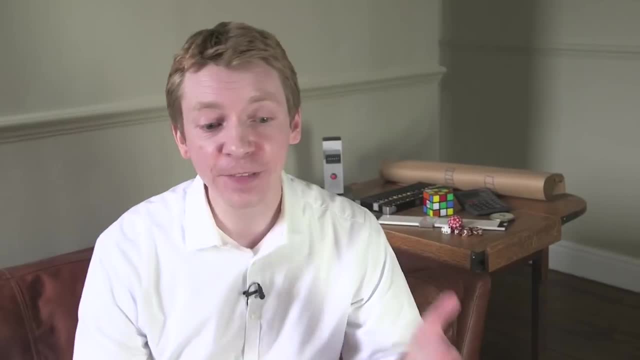 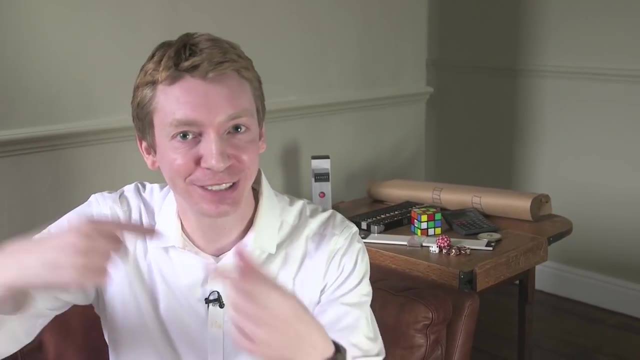 isn't enough to explain the bias that we found. If that's the case, then we're looking for prime gaps less than ten. right, That means you know the next one is less than ten. So it's you know you're going for the prime ending with a one next, or prime ending with: 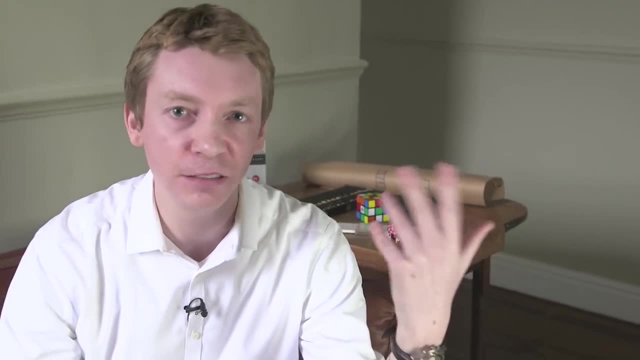 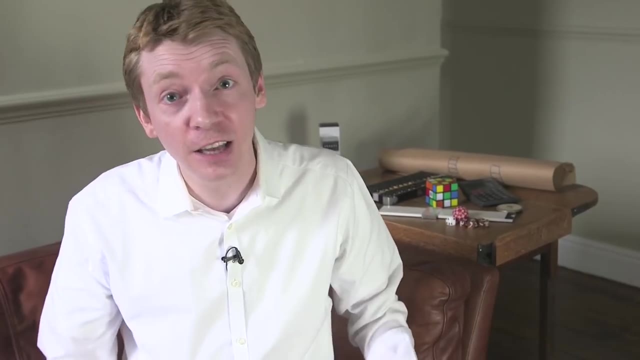 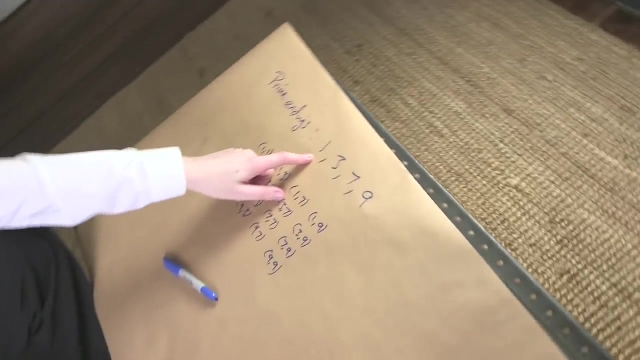 a three next, And prime gaps less than ten are not that many, And so that's not enough to explain how biased this is. The bias is bigger than that, So that's no good. Another explanation might be: I said that these prime endings 1,, 3,, 7, and 9, if this was a random. 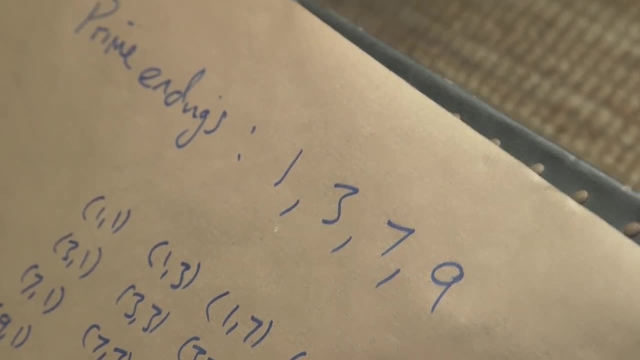 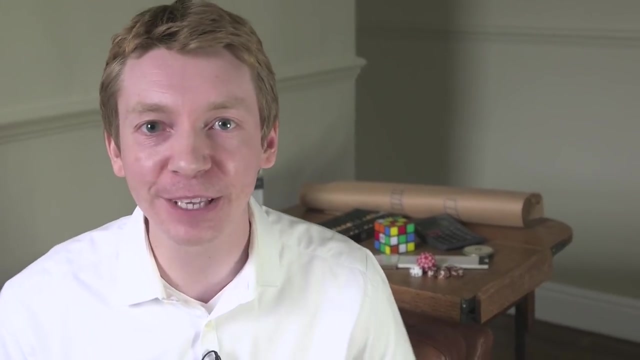 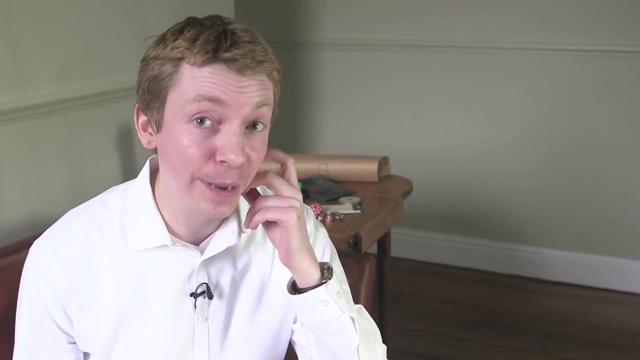 thing they should be appearing a quarter of the time each. Maybe the explanation is that that's not a true thing. Maybe the bias comes from the primes themselves, And that doesn't work out either. There is a slight bias in the primes, And it's something we know about. It's called 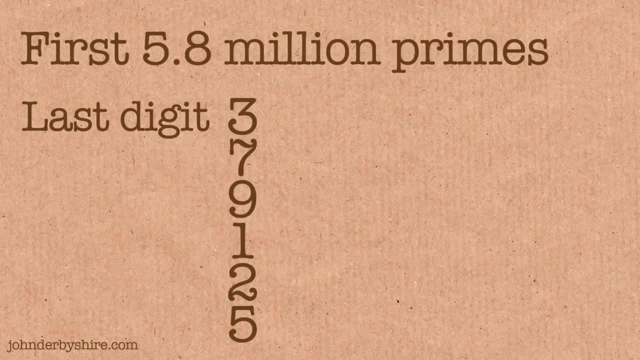 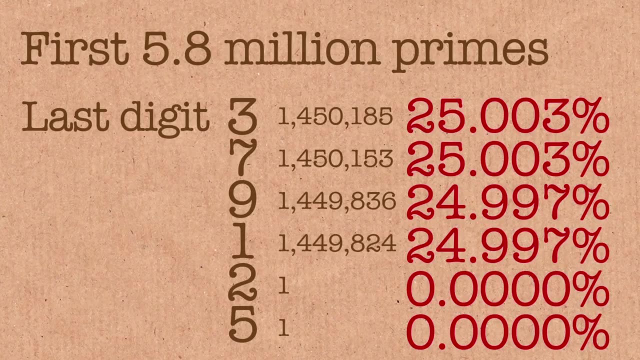 Chebyshev's bias, And it says that primes ending in three, 3 and 7 are slightly more likely. That is something we know about. We know why that happens and it's such a slight thing. It's not enough. 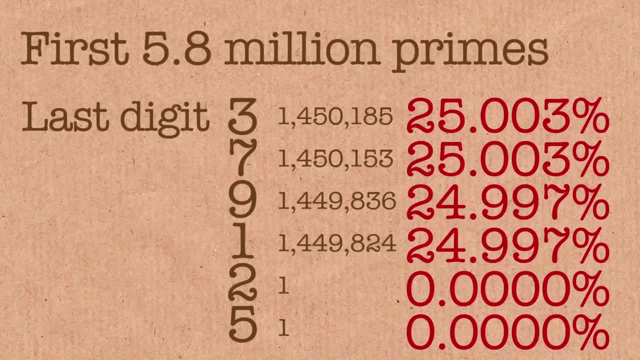 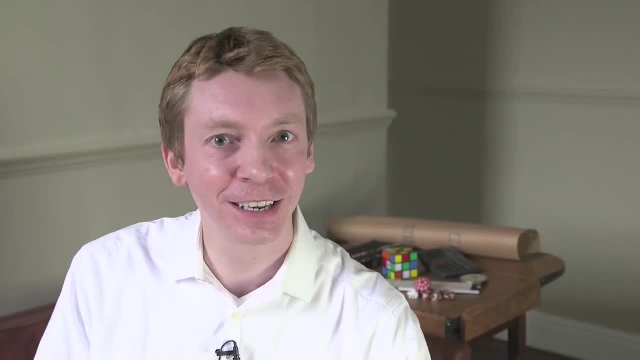 So there's this known bias in prime number endings. So under that assumption, the pair 3, 3 and 7, 7 should turn up more often, right, And the complete opposite is true, In fact. 3, 3 and 7, 7 are the least likely. 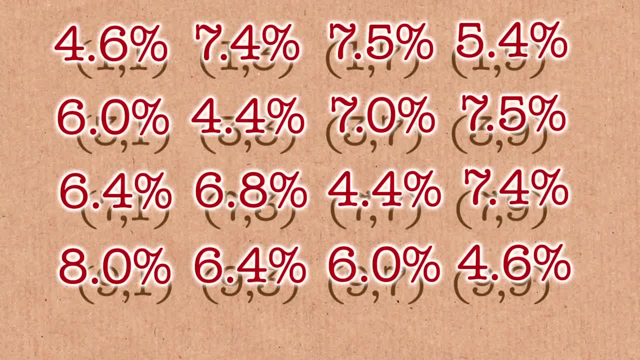 that are turning up, which is the exact opposite of what it should be, And 9, 1 are actually the most common pair, which is not what it should be at all. Okay, maybe, oh, maybe. it's just a base 10 thing. 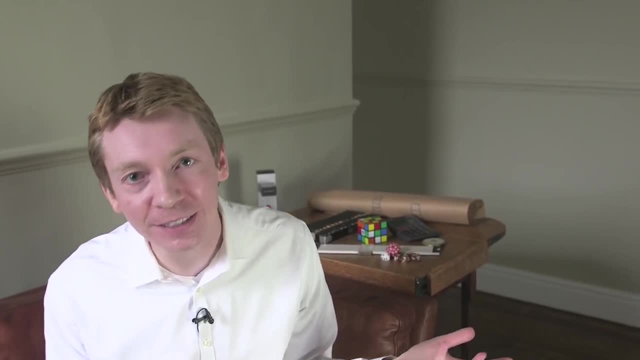 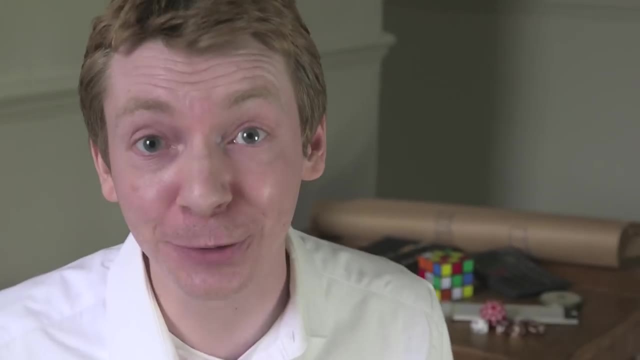 You know base 10, who cares about base 10, right, If it was a fundamental property of primes, it would happen in any base, and it does. That's what they found. So they checked it in other bases and they found the bias. 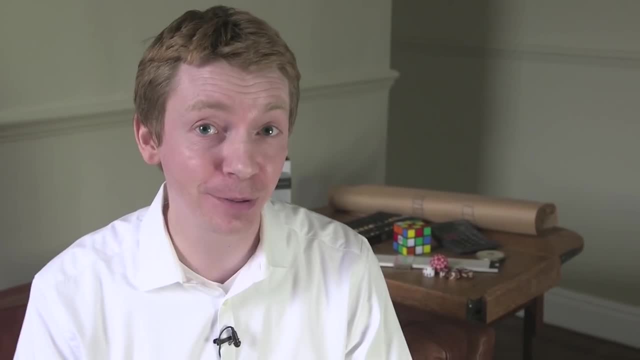 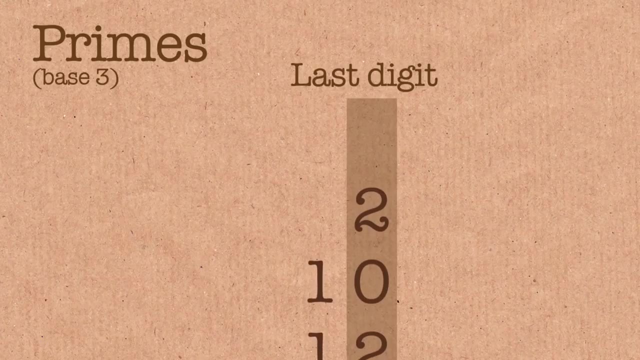 The bias is still there, So it appears to be a fundamental property of the primes. For example, if we drew it in base 3, it will only end with a 1 or a 2, unless it's 3 itself, right. 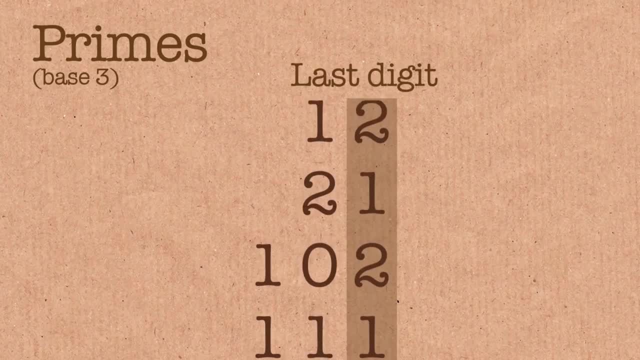 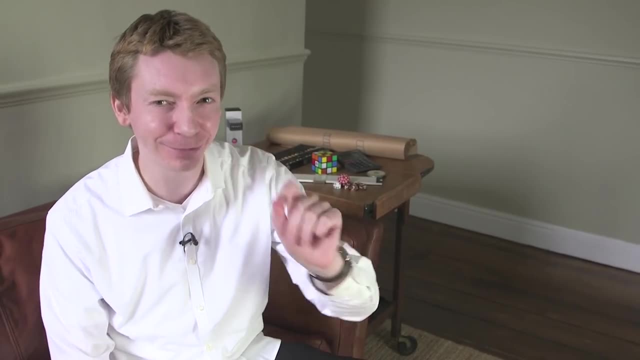 We can ignore that one. You've got two endings. They should turn up about 50% of the time each, which is about right. Again, Chebyshev's bias says it's a little slight bias towards the 2, but it's tiny. 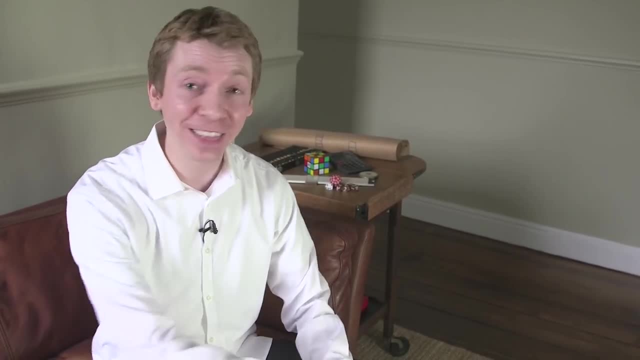 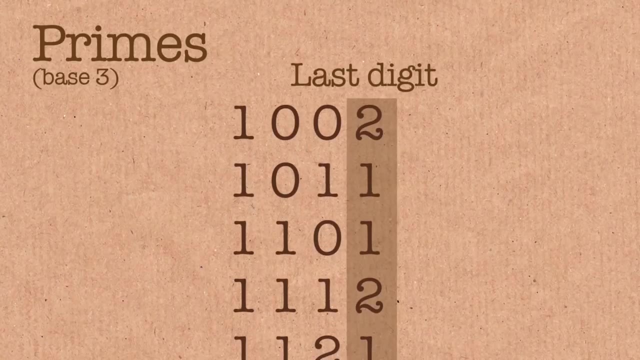 It's pretty much 50-50.. It's pretty much a coin toss. In fact, that's what inspired this investigation. The guys who did this investigation were thinking about coin tosses and so they thought: well, primes in base 3 are like a coin toss. 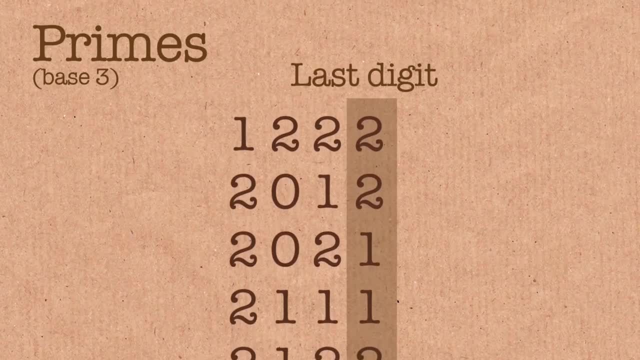 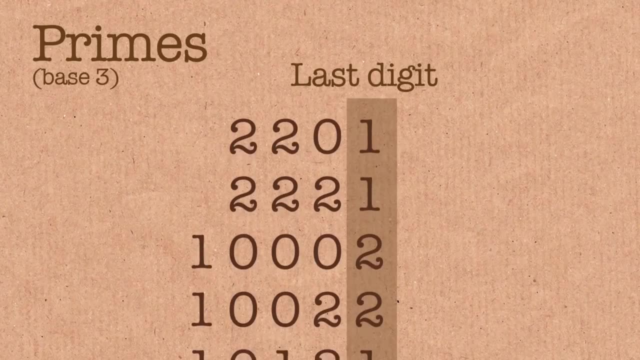 Let's just see if that does the same thing, because that's a random event. And then they found this completely different thing: that there's this skew that primes don't like to repeat themselves, And that's not something that would happen in coin tosses. 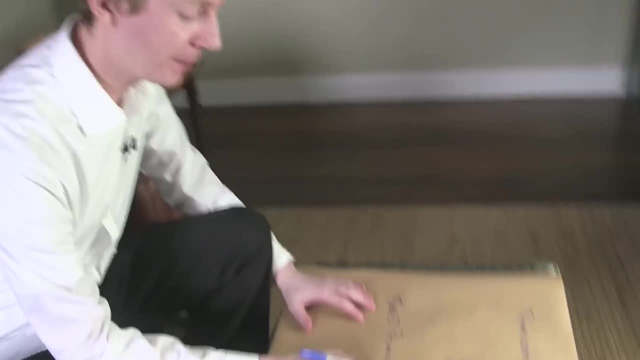 So if we did it in base 3, we would have four prime endings, wouldn't we? We'd have 1, 1,, 1,, 2,, 2,, 1, and 2, 2.. And again, they found the same thing. 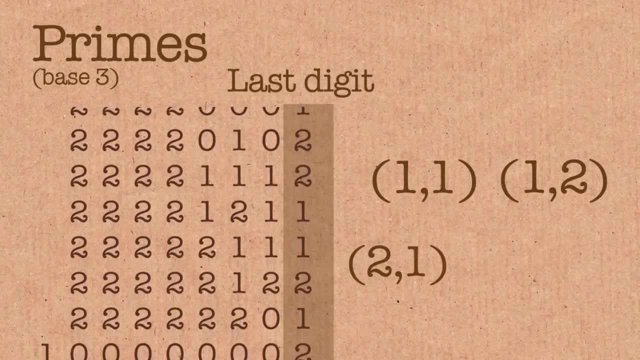 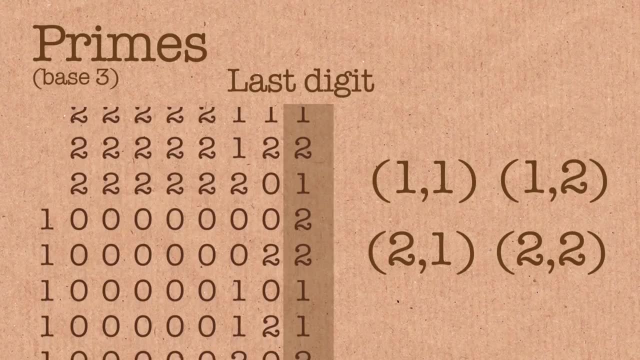 These ones with the repetition are the least likely to occur. They looked at the first million primes And if you look at the first million primes then they should all be equally likely. Should all turn up a quarter of the time: 250,000.. 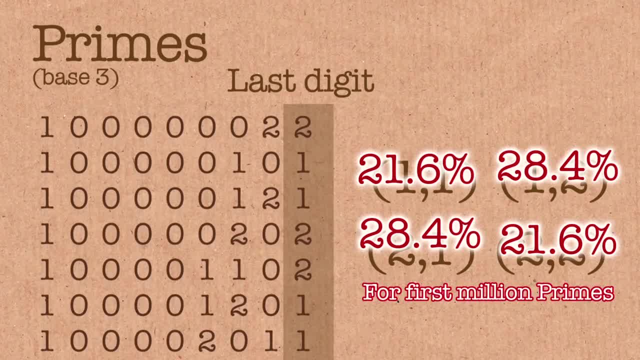 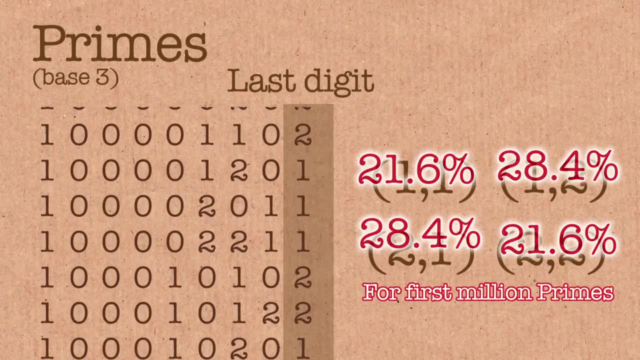 But no, they didn't get that. So these ones with the repetition were less than 250,000.. The ones without a repetition were more than 250,000.. So the mathematicians who have been investigating this have tried to come up with an explanation for this. 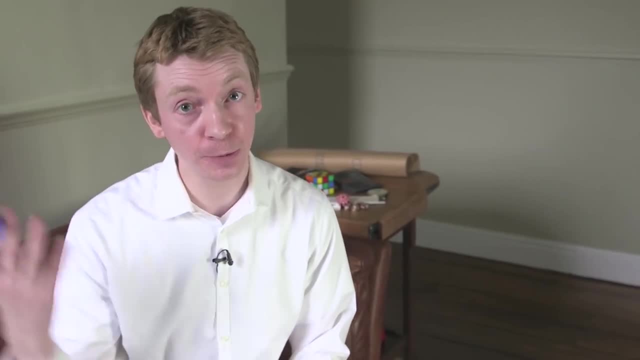 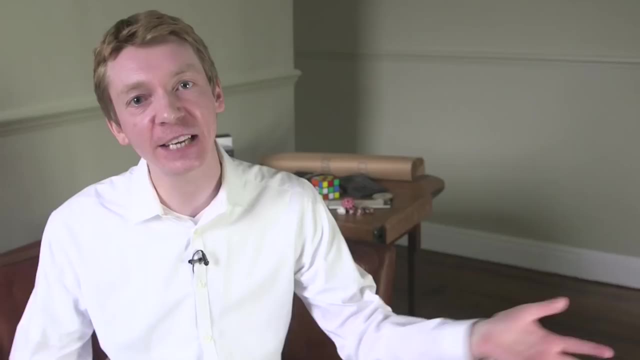 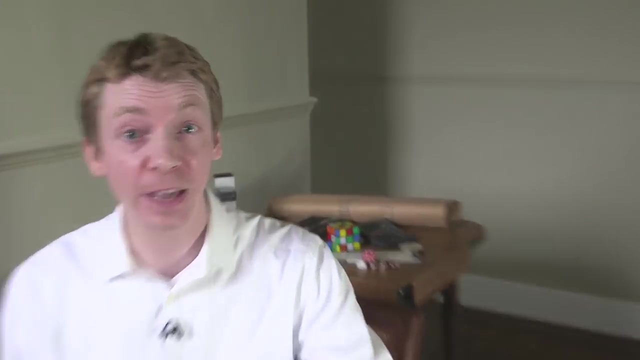 And their explanation relies on a conjecture that goes back 100 years. It's a conjecture by Hardy and Littlewood And they had a conjecture about the density of primes, how many primes you can find in patterns, So you can consider all kinds of patterns like twin primes. 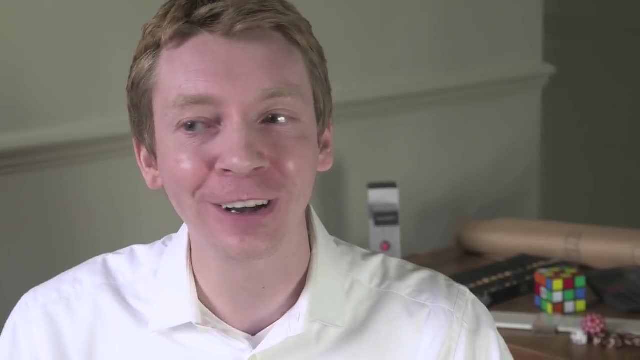 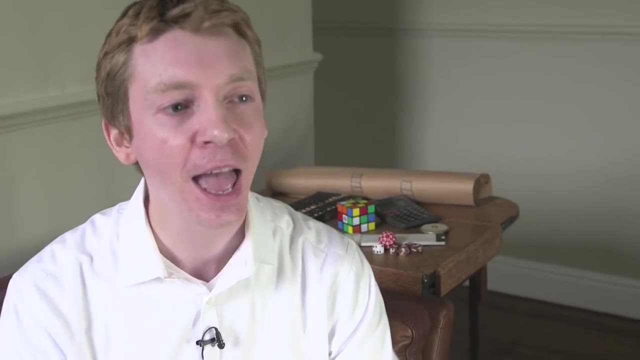 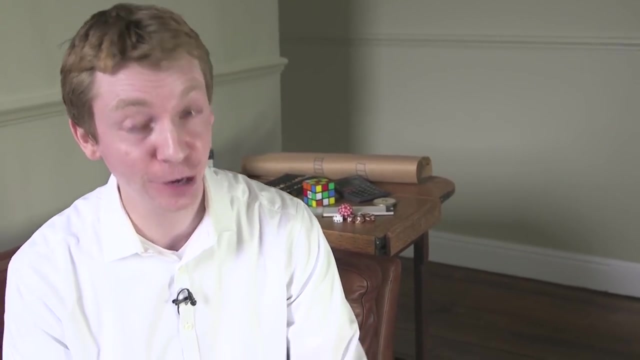 That's a pattern. Or cousin primes, which have gaps of four, Or sexy primes- You have gaps of six. So they had this conjecture about how many of these you should find, And the conjecture has not been proven. There's a lot of evidence that supports that. it's true. 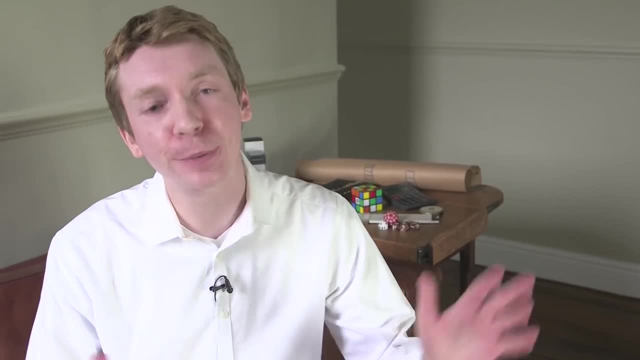 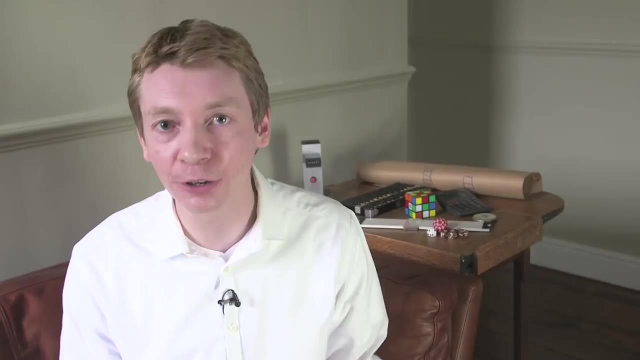 So if you look at the numerical evidence, it appears to be true, but it hasn't been proven. So the mathematicians looking at this pattern used a modified version of that conjecture And they came up with a formula that they think might explain this idea. 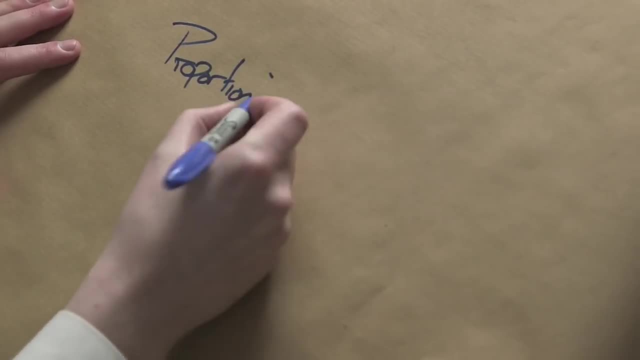 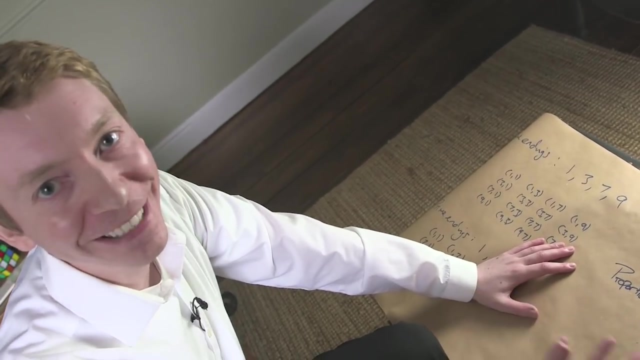 So the formula was: So the proportion of this pattern? Let's say you've got prime endings a and b. So if we're doing it in base ten, this could be one-one or three-seven, or nine-one, And so we're looking at the proportion of these endings. 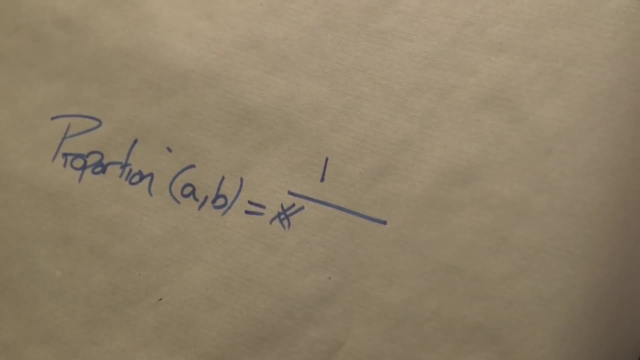 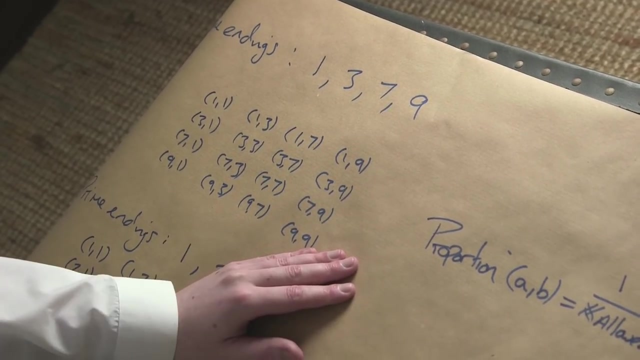 And they came up with a formula. The formula was one over the number of allowed endings, So this is like 1: 16th from what I've been doing in base ten, Right? So when it's equally likely, these are the allowed endings there, 16 of them. 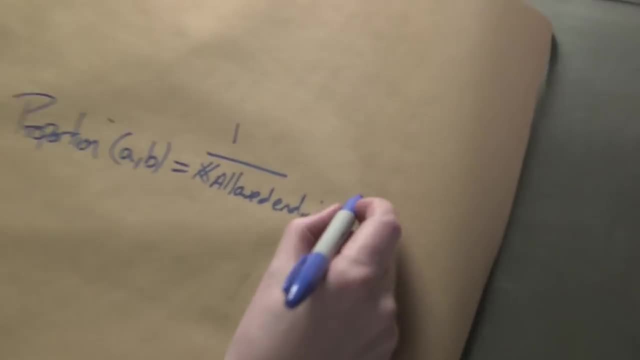 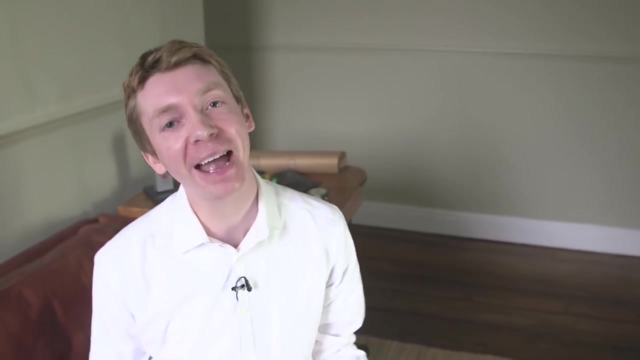 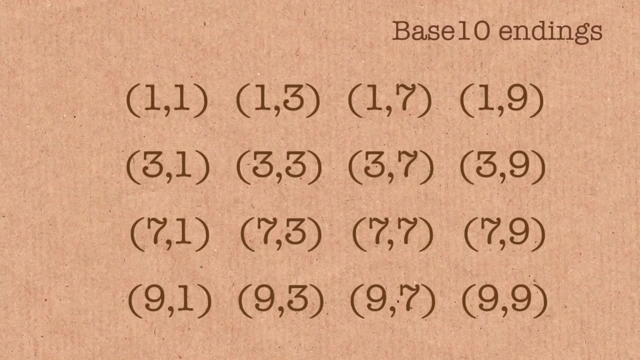 So the proportion is 1 over the allowed endings multiplied by a thing. Right, and what is this thing? OK, that thing depends on if that pattern repeats. If you've got a equals b in that formula, If a equals b, that will affect what that thing is. 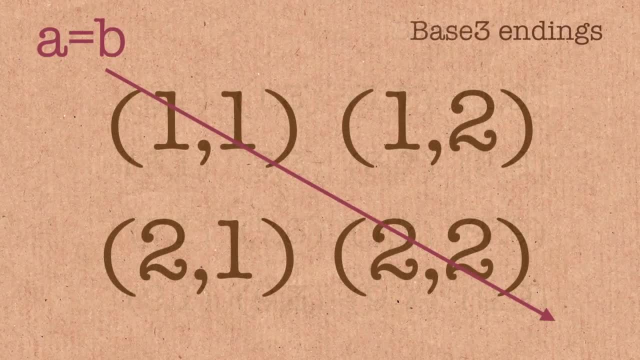 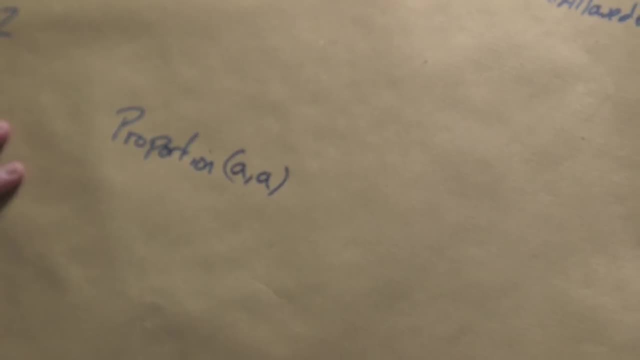 I'll show you what it looks like in base 3.. It's kind of OK in base 3.. We're looking at proportions of these endings. If they're the same, like this: a, a. so that would be in base 3 the 1, 1 endings and the 2, 2 endings.